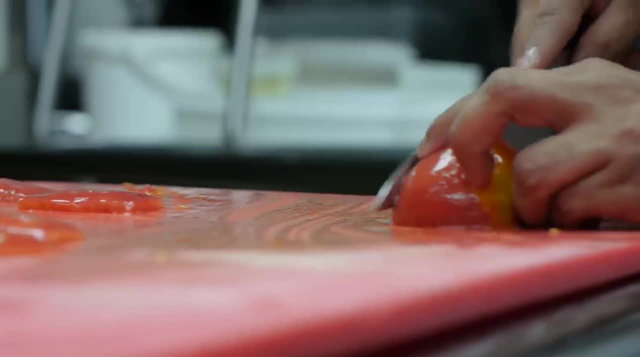 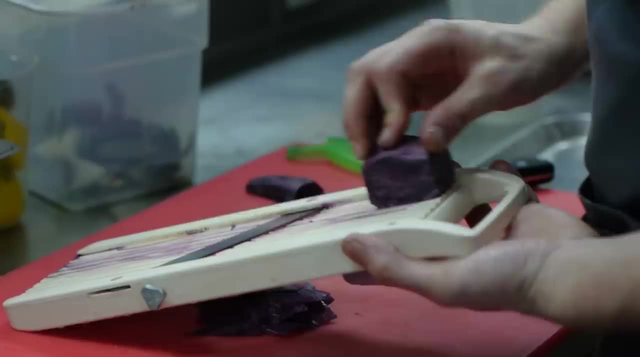 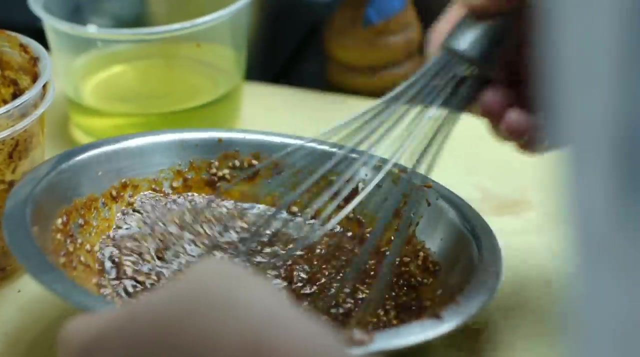 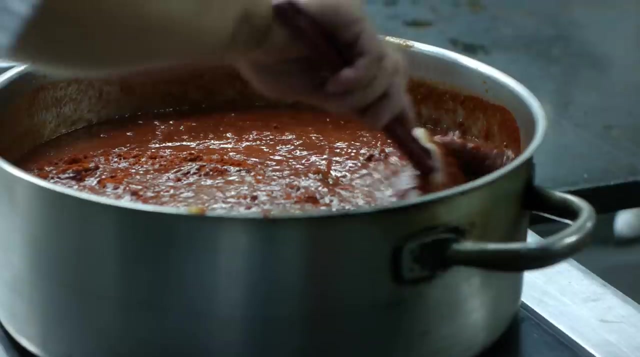 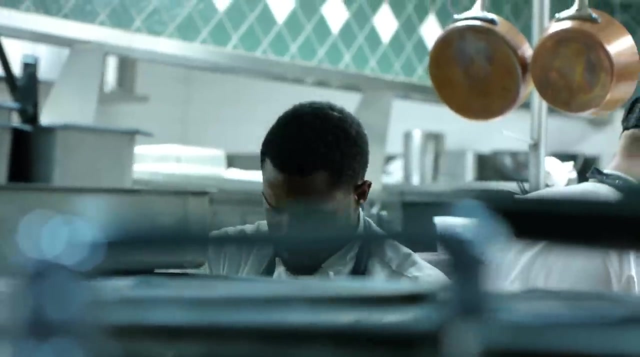 prepping. We have to get fish to bone, tomatoes concasayed, the sauce is simmering. all this has to be ready before service at 6 o'clock. Working in the kitchen is one of the hardest jobs I've had in my life. 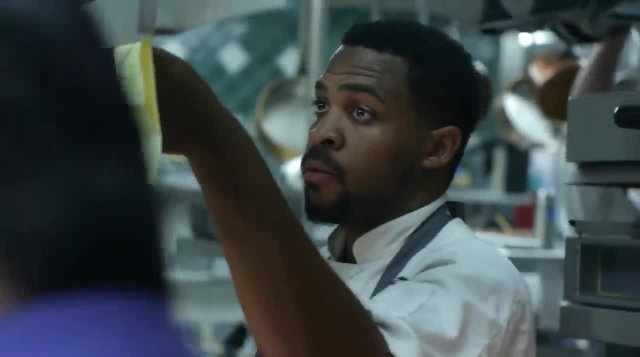 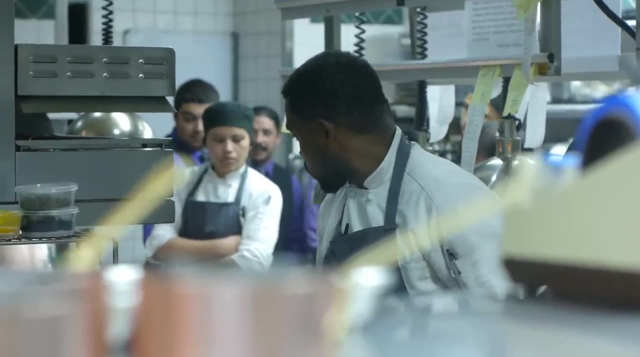 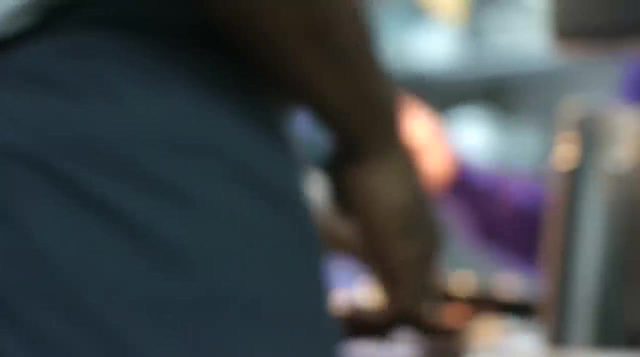 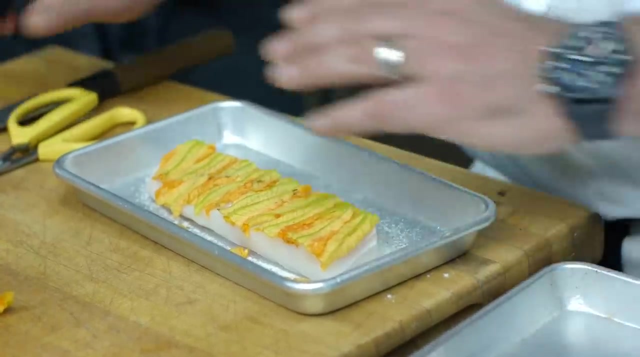 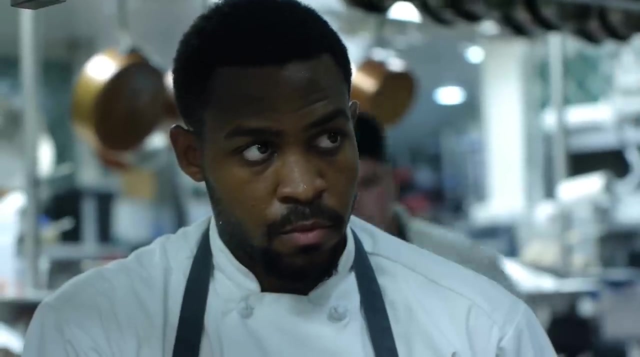 You're under this constant stress and on top of that you're working long hours, you're on your feet all day and it's just completely physically and mentally straining and most people can't handle it. But I love it. Chef Josiah Citron is one of the most renowned and respected chefs in LA, and it was only 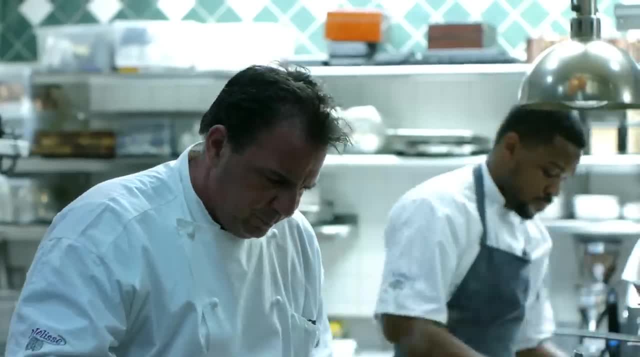 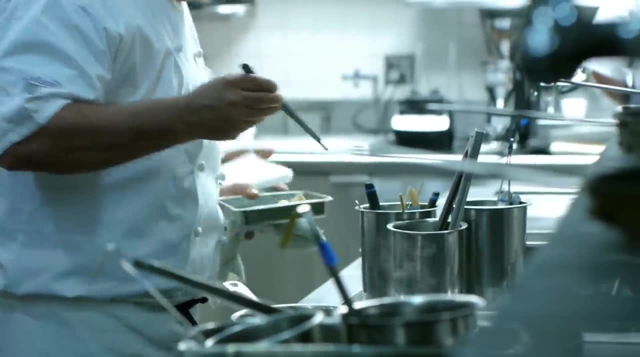 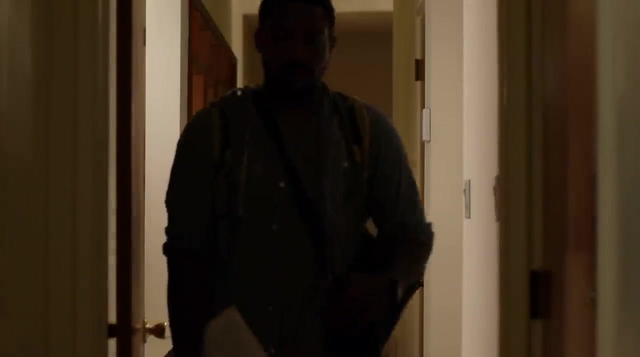 natural that I wanted to come work for him. He's almost like the epitome of an old man, An old school French chef relocated in the US. he has that passion, that drive and intensity that you come to expect from great chefs like himself. 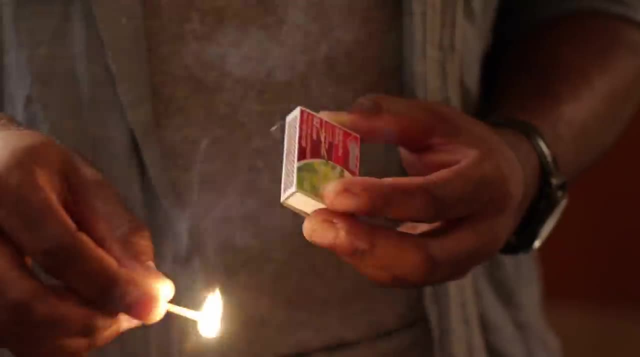 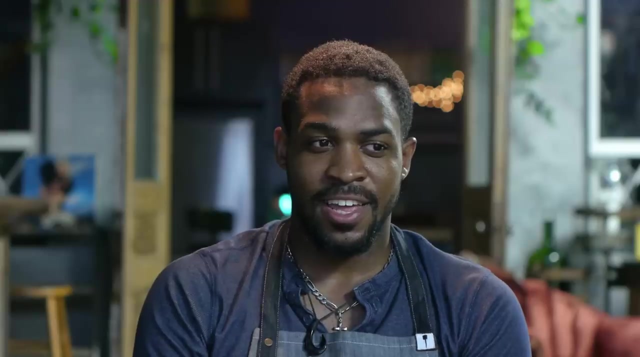 One day I was in the kitchen and I was scrambling eggs and this memory kicked back to me from my grandmother and how she taught me how to properly scramble eggs when I was a little kid And she was explaining how you use a spoon to stir it and cook it really gently, so that 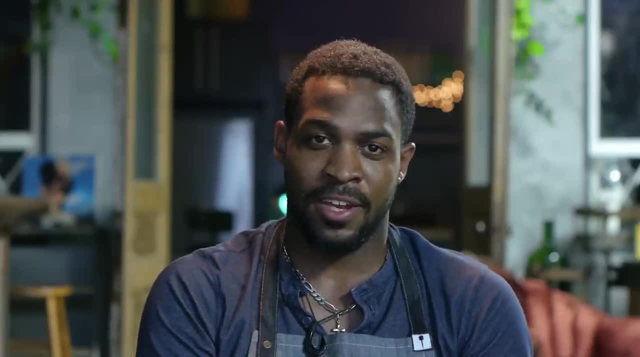 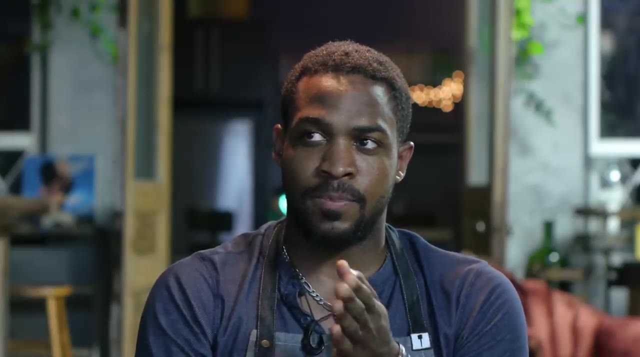 the texture comes out nice And it's actually like a classical French way of cooking And I have a southern grandmother. it was kind of weird And it was like little moments like that that I think back, that kind of directed me to cooking that I didn't really realize until now. 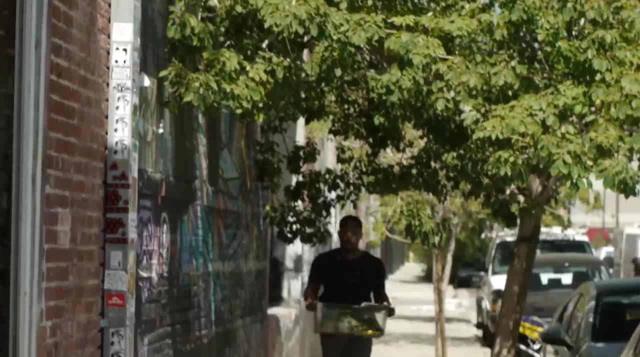 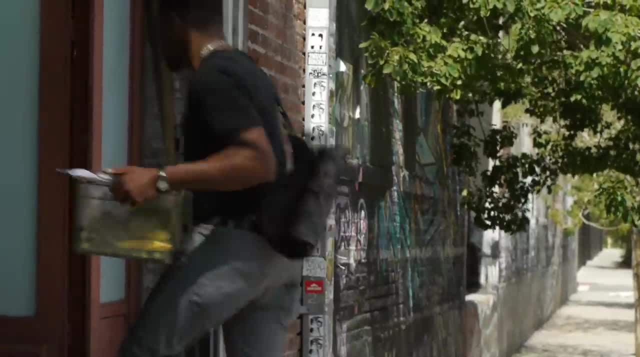 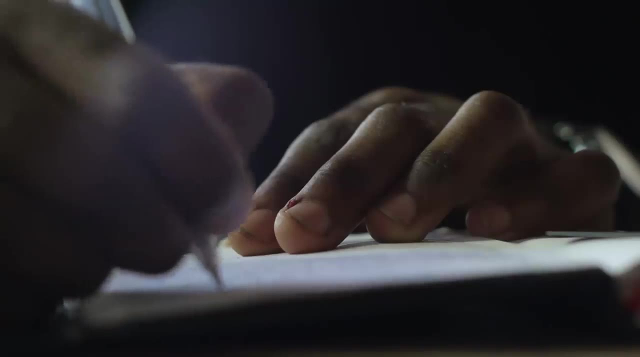 If you want to be a chef, you can't wait around for someone to hand it to you. You almost have to take it. Hosting pop-up dinners have given me and my friend Gary a chance to not only be a chef, but to not only showcase our skills, but to do what we're trained to do: be a chef. 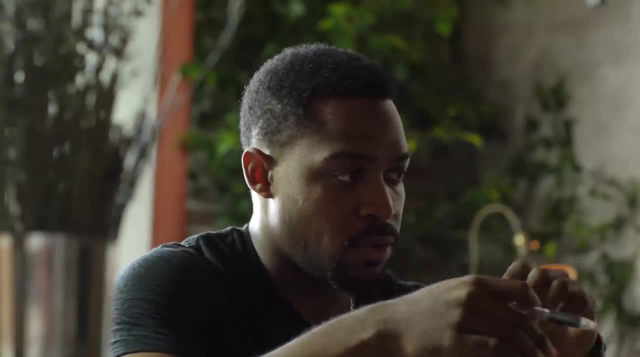 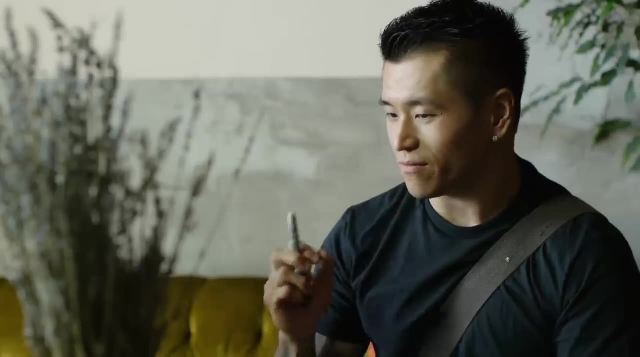 For the oyster dish. I was thinking: right, we have those nice clear bowls, we'll put the garnish in the middle and then pour the gazpacho, so it comes like two-thirds of the way up. I brought a fish tank bubbler and instead of making foam with the frother, let's do.